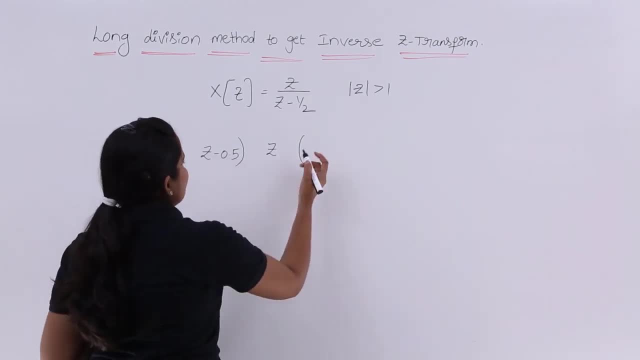 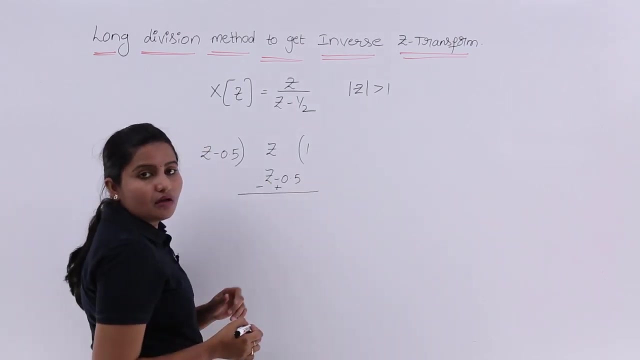 my convenience. I am considering like 0.5. So here it is. goes like this. So it goes for 1 time. So z minus 0.5.. So I am going to change the signs: minus, plus already. minus is there. I am writing plus here. plus is there. I written minus Once I changed. 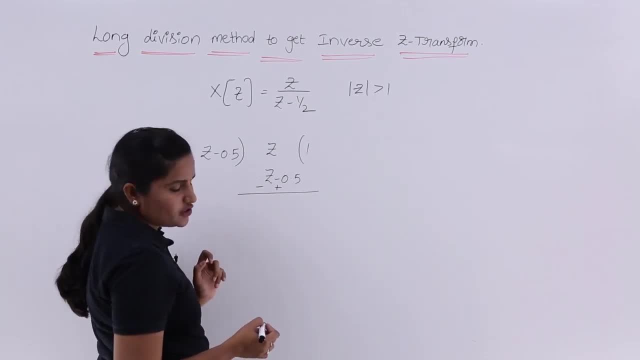 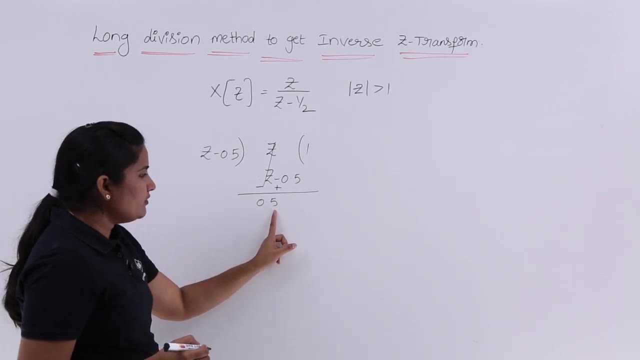 the sign. in every step I need to go for sign change. So z, z is going to cancel. I will get 0.5 here. So see here: this 0.5 I need to get rid by using z only. Please keep in mind that is the only point. So here I am multiplying that 1 time that. 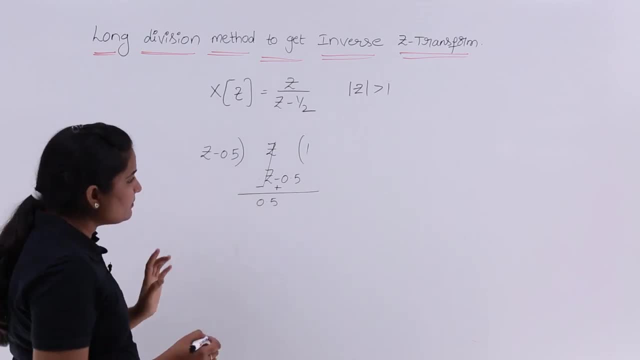 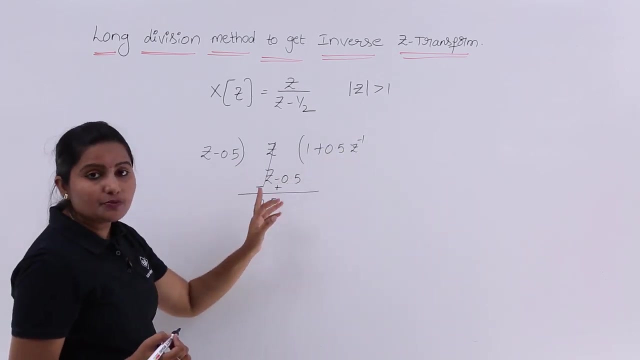 means z into 0.5 z inverse. for example, if I multiply like this: 0.5 z inverse, 0.5 z inverse, if I consider, then z into z inverse will vanish and the remaining is 0.5. that is very important. 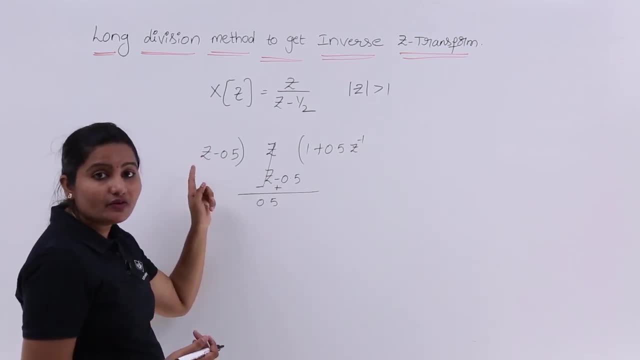 We should take every step by taking the reference of this maximum polynomial of z. that is very important point. So you can make z minus 0.5 into 1 also, it is going to cancel this 0.5, but we cannot take like that in this method. So you need to take reference of. 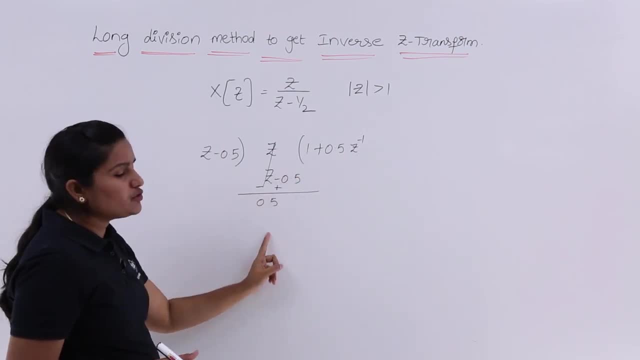 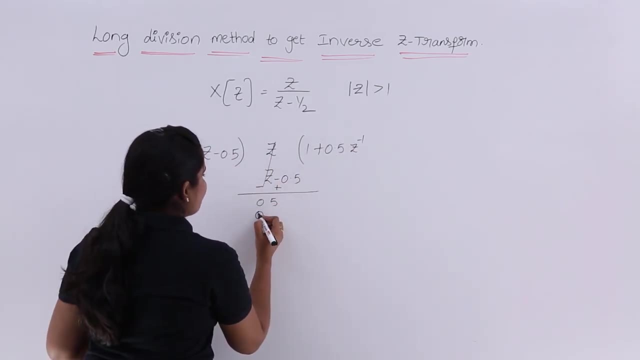 z every time. with this z only, you need to evaluate each and every step. So if I consider 0.5 z inverse time, then this z will become 0.5.. So 1.5 z inverse 0.5.. So L is going. 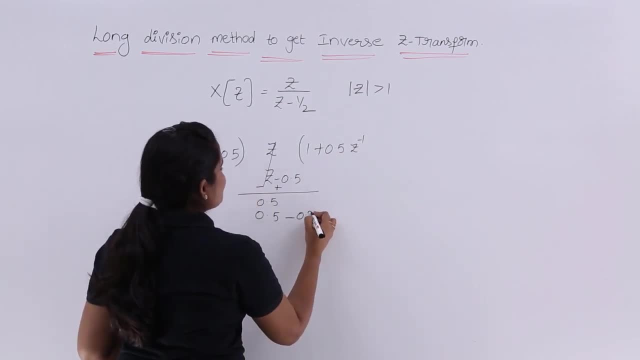 to be 0.5 z inverse. So I am going to write 0.5 z inverse 1 by z inverse. So if I consider So minus 0.5 into 0.5, 0.25 z inverse. again I am going to sign change. So these two are. 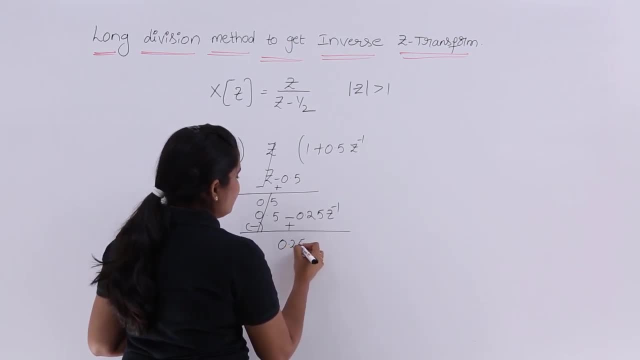 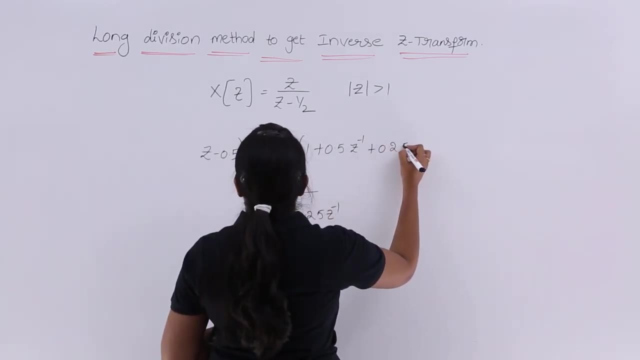 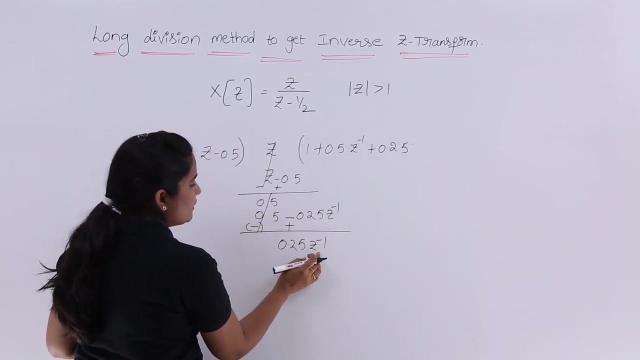 going to cancel. remaining is 0.25 z inverse. Again, to get 0.2 z inverse, how you will take 0.25 z inverse or how much you need to consider already here. z is there, you need to get 0.25. 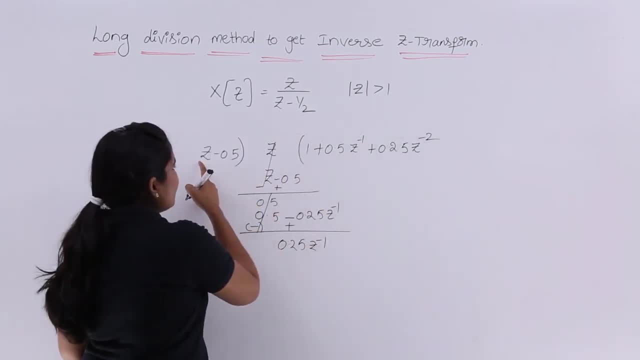 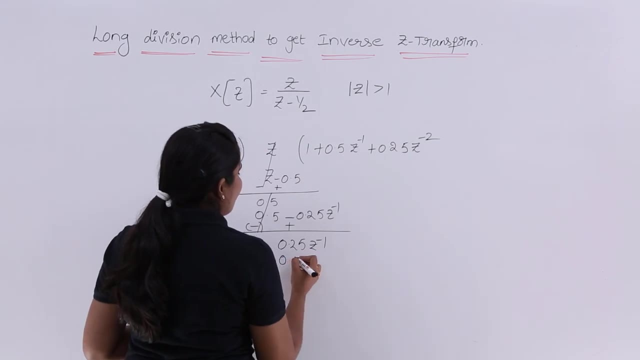 z inverse. So that is why z power minus 2.. So if you multiplied z into 0.25 z power minus 2, you are going to get 0.25 z inverse. So here 0.25 z power z inverse minus 0.5. 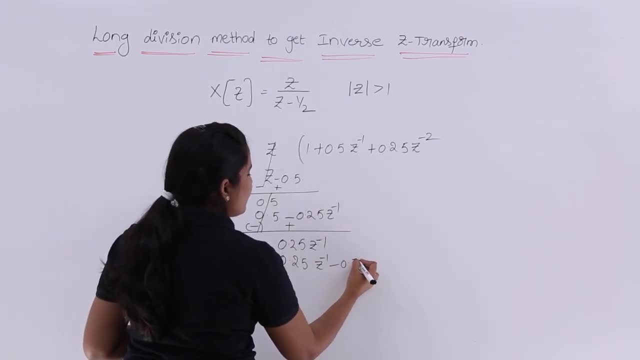 into 0.25. you are going to get some value 0.5 into that means 1 by 2 into 1 by 4. 1 by 2 into 1 by 4 means So 8, 1 by 8 into z power minus. 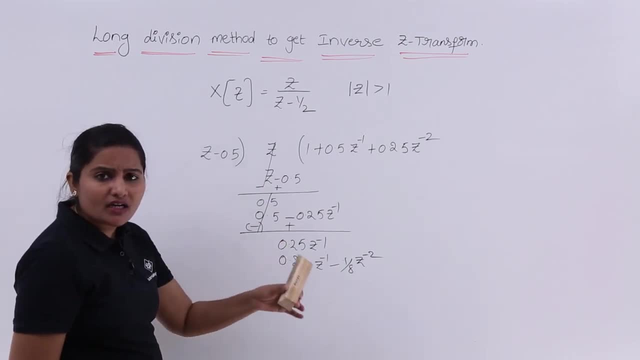 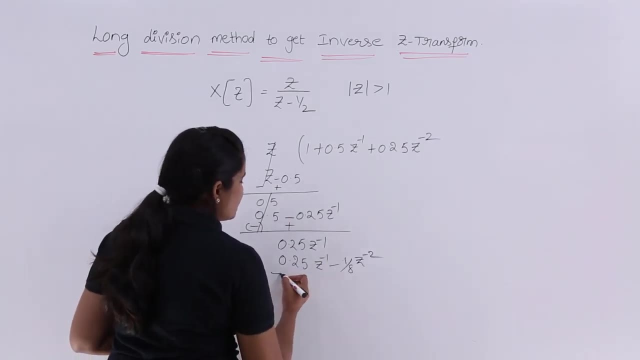 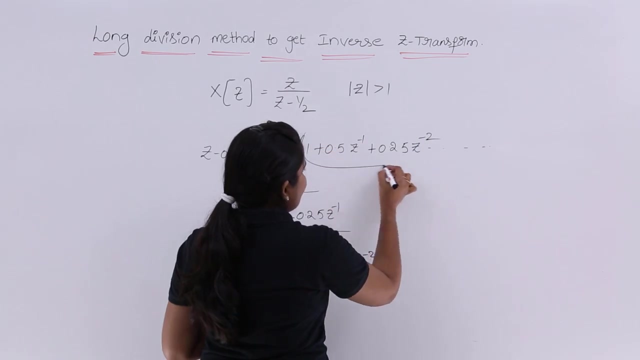 2. that means 0.10 something, 1, 2 something you will get, 0.12, something you will get. So here, 1 by 8, z power minus 2. this process will continue. you are going to get continuous values here. So whatever you got as your coefficient that you need to consider and 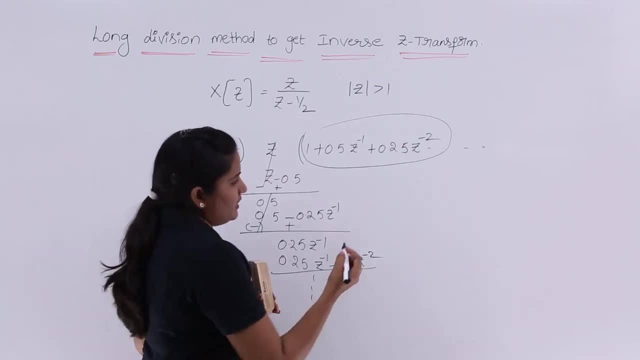 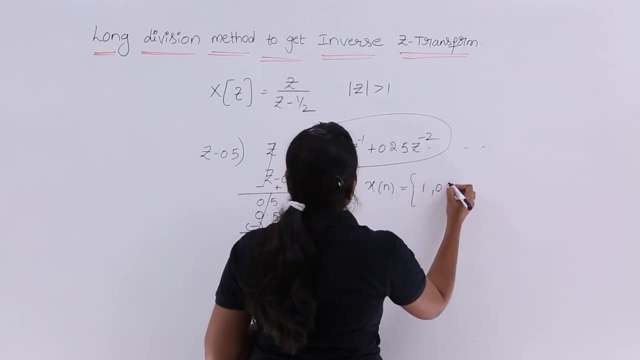 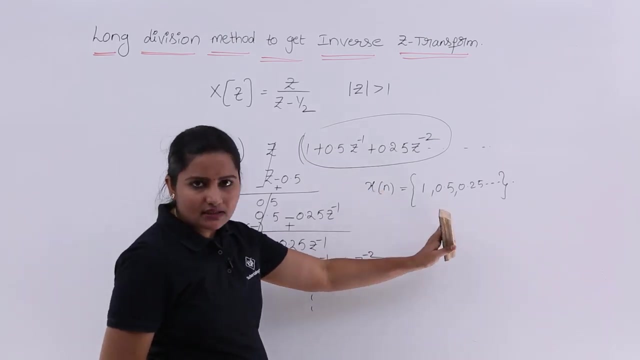 you need to consider the coefficients as x of n. So here x of n is equivalent to: So 1 comma 0.5 comma 0.25, and so on. So this is your signal. this is inverse transform of this. 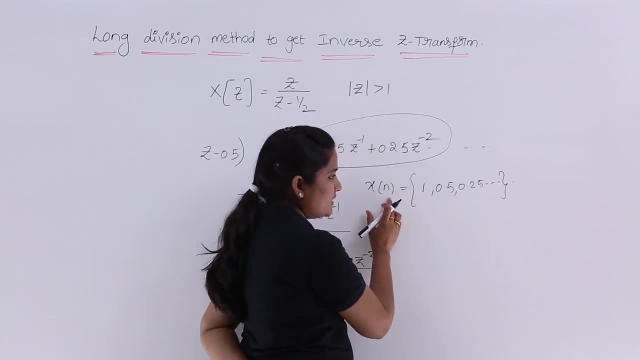 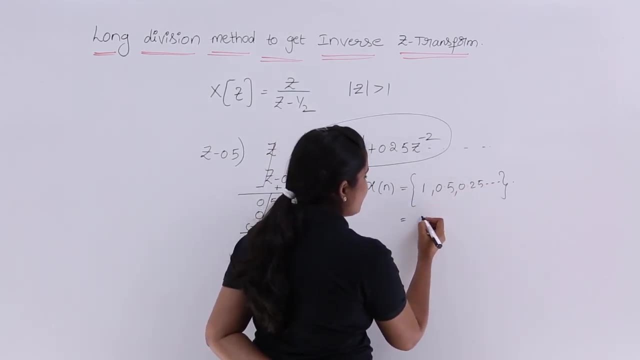 So here you can observe, if you want to write in terms of n, if you want to write this summation, So you can see, this is all positive sided, I am going to write like this. So I am going to write like this: 1 by 2, whole square. So I am going to write like this: 1 by 2, whole. 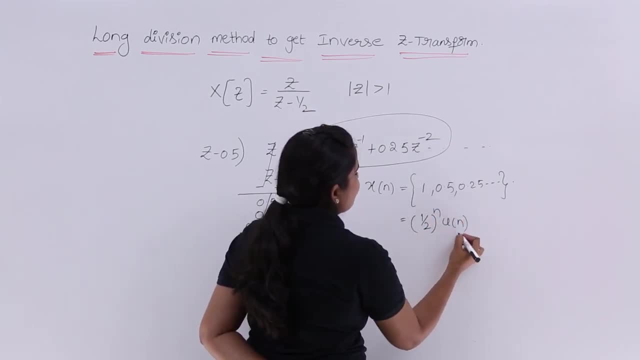 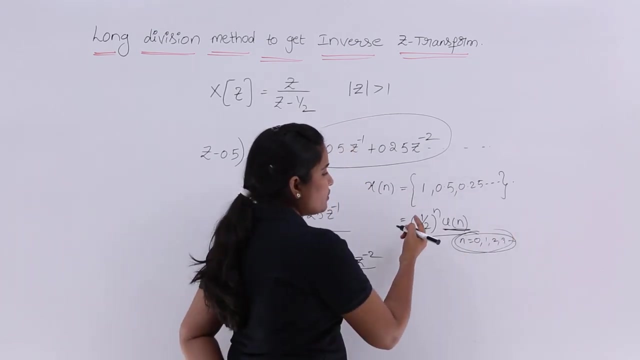 power n? u of n. I am going to write like this why? because if I substituted 0, where n is equivalent to 0, 1, 2, 3 so on, u of n itself represents this. no need to write this. So when n equivalent to 0, 1 by 2- whole power. n means 1 by 2 whole power. 0? u of n is equivalent. 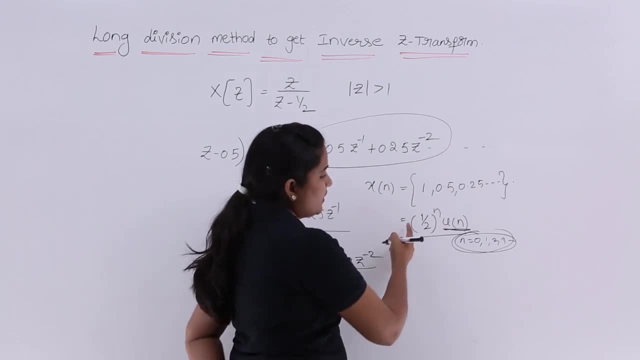 to 1.. 1 when n equivalent to 1. 1 by 2 into u of n, that means 0.5 into 0.5, into 0.5, into 5, into 1, 0.5.. So 1 by 2, whole power 2. 1 by 4, that is 0.25. you are going to get the same. 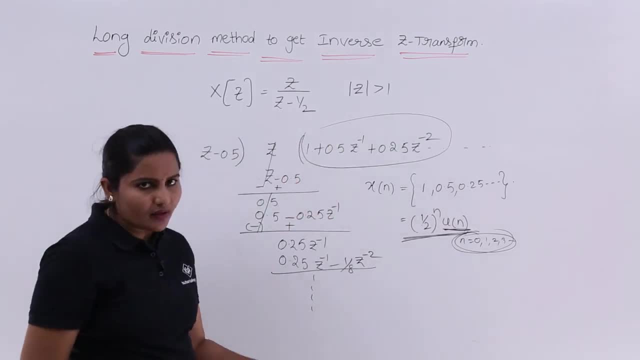 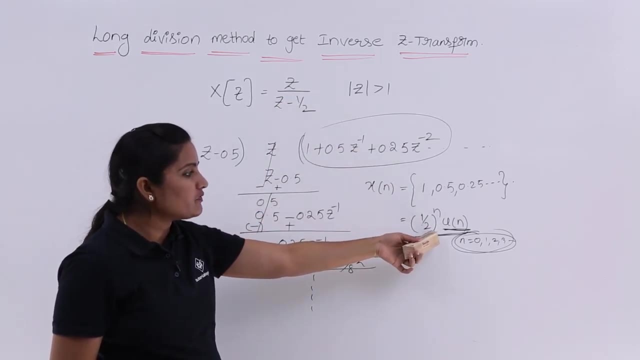 So the inverse transform is 1 by 2 whole power? n? u of n, by generally method, also generally. also, you know, the inverse transform of z by z minus 1 by 2 is 1 by 2 whole power? n? u of n. So like this way, like by using this long division method, you can calculate the inverse. 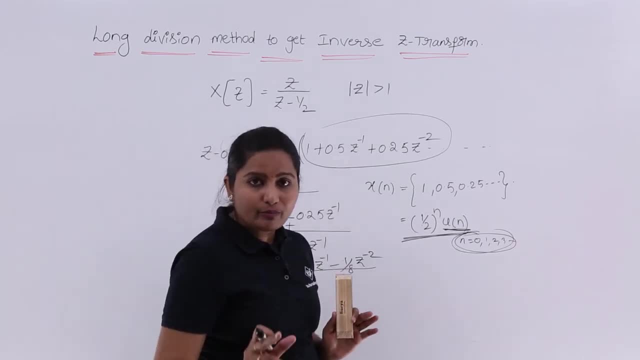 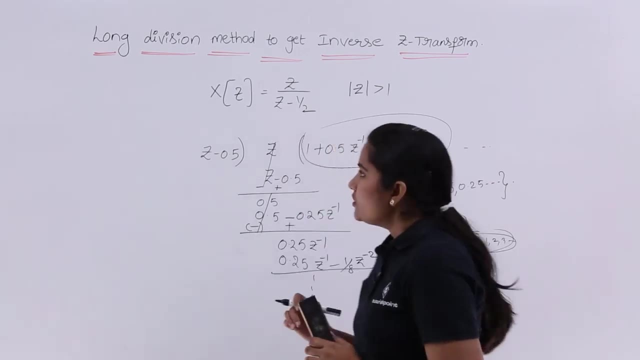 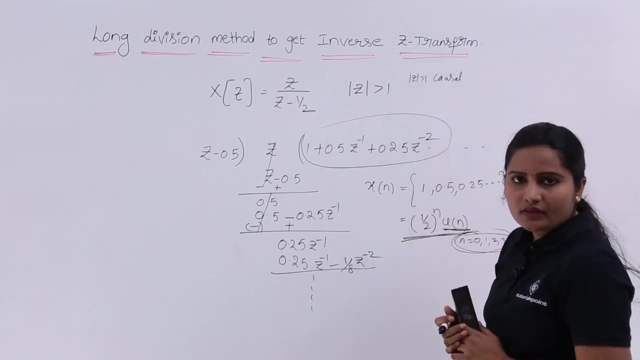 transform. Now here I will give you two important points when you are dealing with this long division method: inverse transform. So when system is causal, that means when mod z greater than 1, you need to consider descending powers of z or ascending powers. 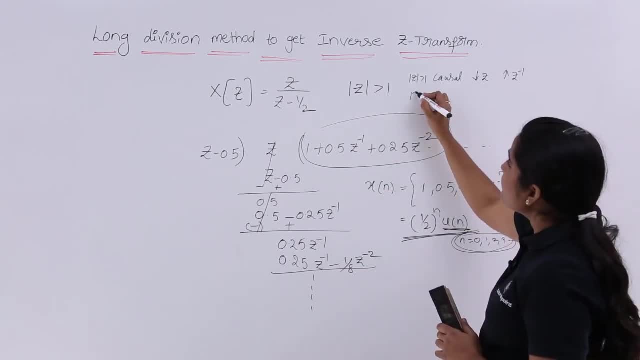 of z inverse. If system ROC is mod z less than 1, that means non-causal. if the system is non-causal, you need to consider the given function in ascending powers of z or descending powers of z inverse. that is very important, So here. 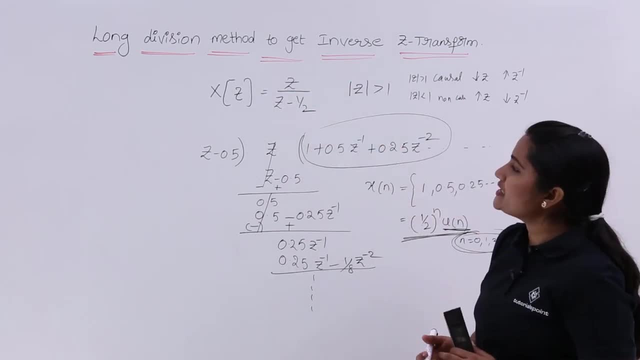 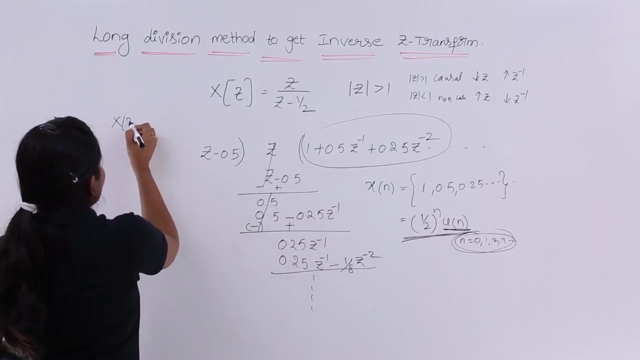 for example, for this system, if you see mod z greater than 1, is there mod z greater than 1? this is a causal system. So we need to consider descending powers of z. I consider z. So any x of z is given like this: x of z is equaling to some z plus z square by z cube. 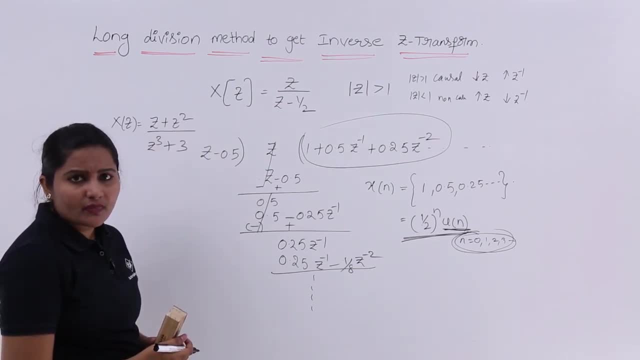 plus 3, like this is given. So how we can consider 3 plus z cube, 3 plus z plus z cube, So like this: they given x of z. So for this also we can go for long division method. but 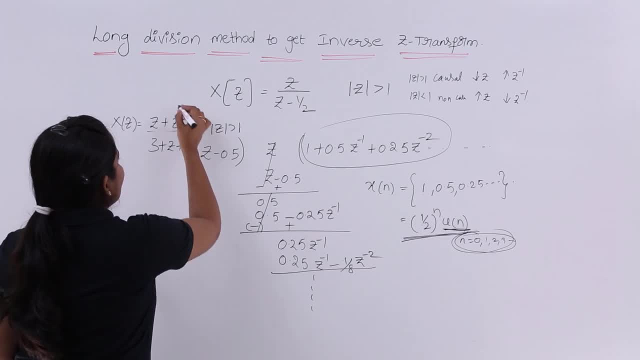 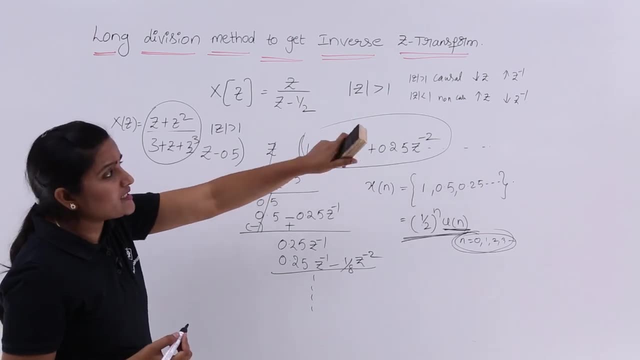 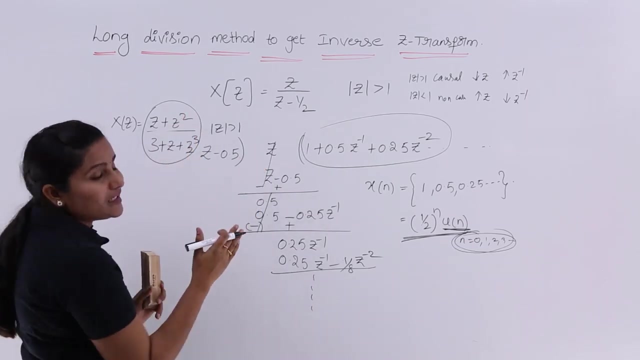 when they said mod z greater than 1. you need to consider this x of z as descending powers of z or ascending powers of z inverse. they given in terms of z. If they given in terms of z, then you need to consider descending powers of z, You do. 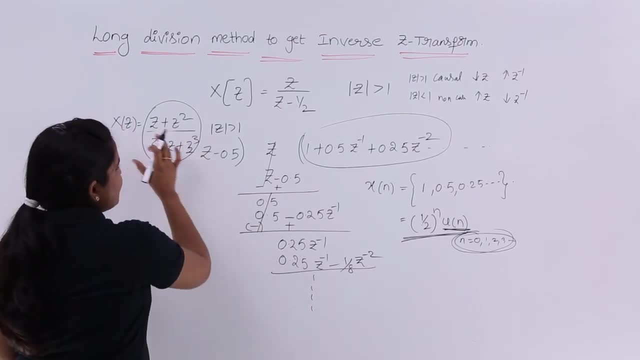 not take like this for a division. do not take 3 plus z cube in division like that. So you just consider this as z cube 3.. Yes, Som though I took that okay. Now, if x of z is greater square plus z, right descending powers of z, z square after z and z cube plus z plus 3. 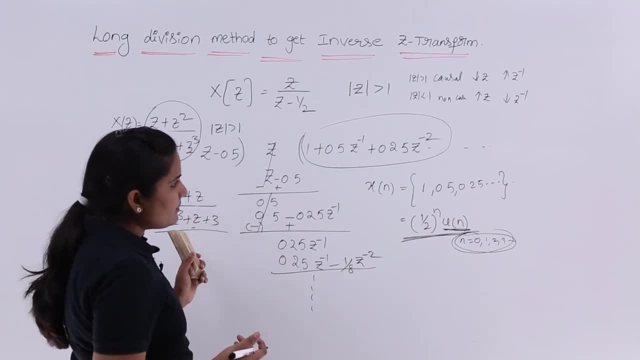 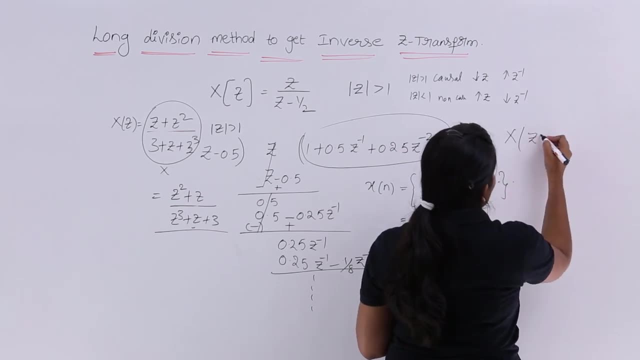 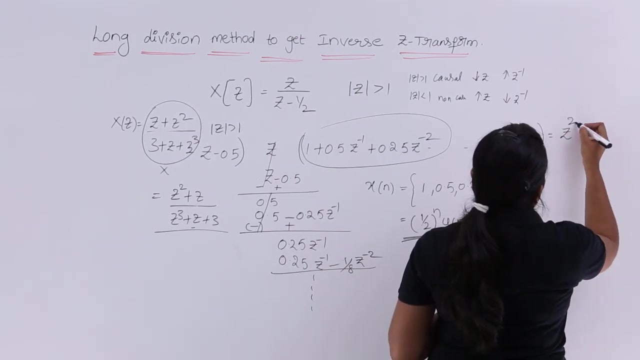 now perform the division. For example, they given like this: x of x of z is equaling to x of z is equaling to z power z square plus z cube, z plus 1 divided by z power 4 plus 2, they given like this and they told the ROC is mod z less than 1.. This is anti-causal. 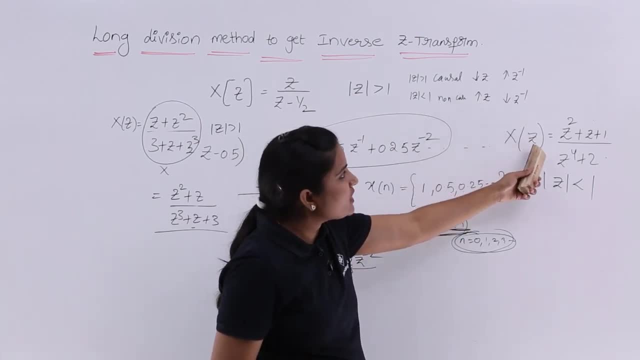 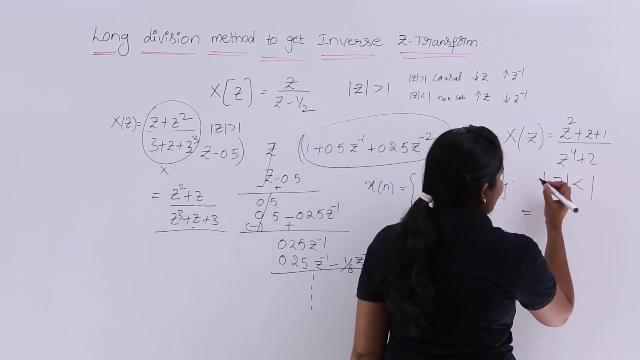 system and given in z domain. So you need to consider ascending powers of z when z is less than 1. And when you are performing the long division method, that means you need to consider ascending powers of z. you need to increase the powers, not decrease the powers they given in decreasing 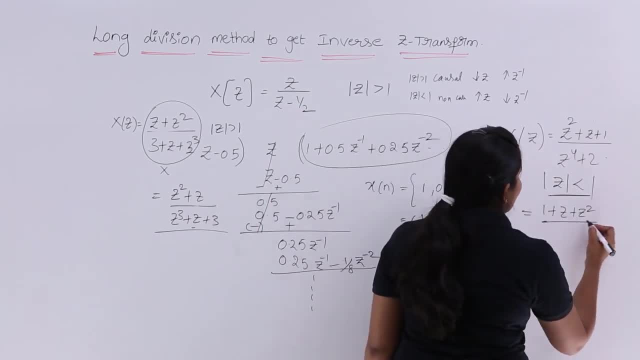 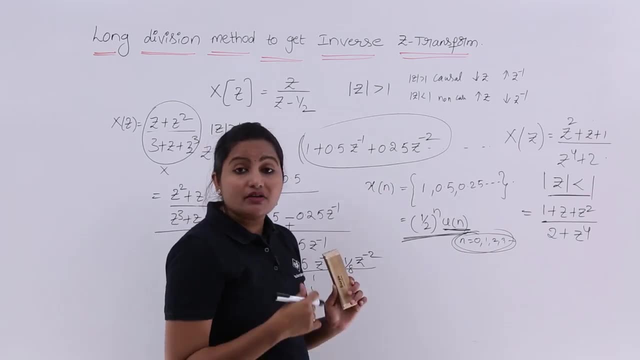 but they given that is a non-causal system. So here you need to consider, you need to rewrite the equation like this, and then you need to perform the long division method, otherwise you are going to get the wrong answers. The general long division method will be like: 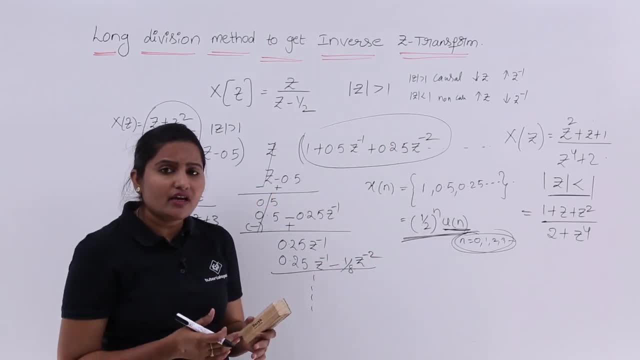 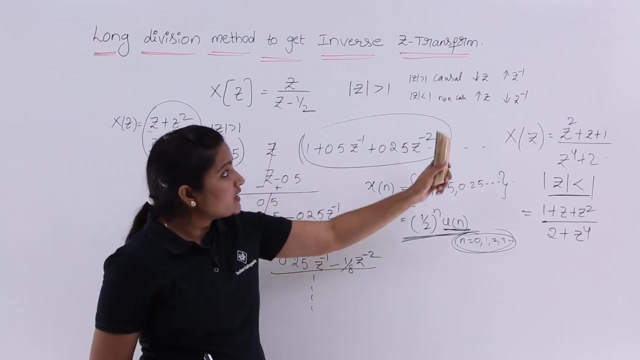 this. So I consider this simple example. you can- you can- get problems in any textbook using long division method. This is a very simple method, but only things you need to follow is So every time you need to take the reference of z, which I considered at first and after that. this point is very important. So if 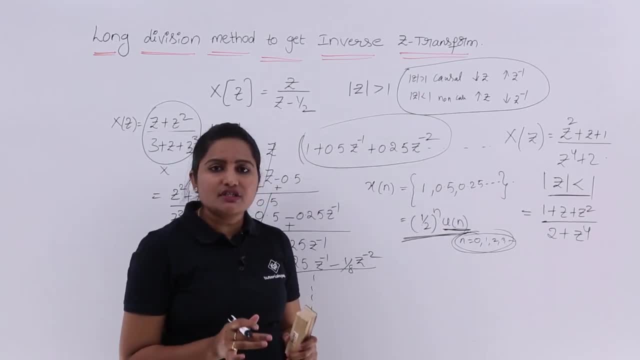 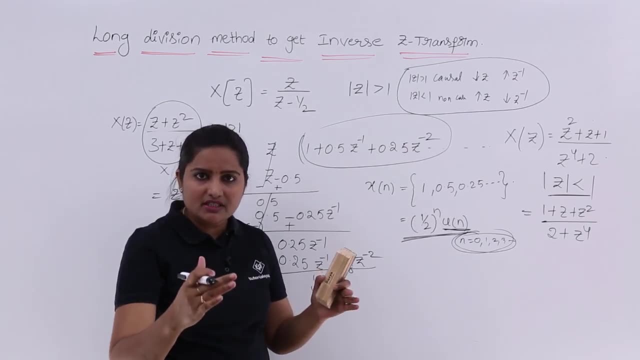 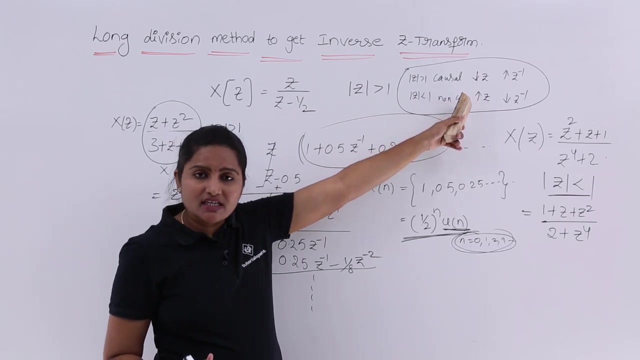 that is causal. you need to consider the equation in descending powers of z or ascending powers of z inverse. If they given in terms of z inverse. the system is given in terms of z, Then you can take ascending powers of z inverse. if this system is given in terms of z, then 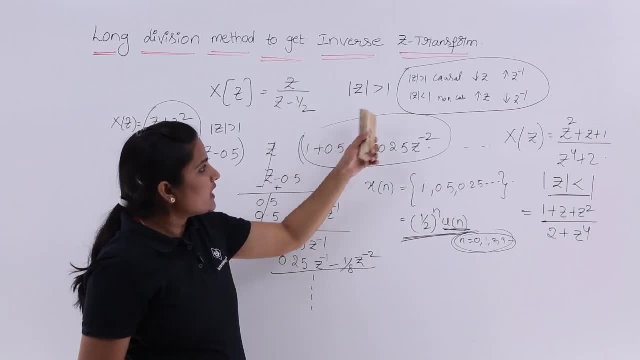 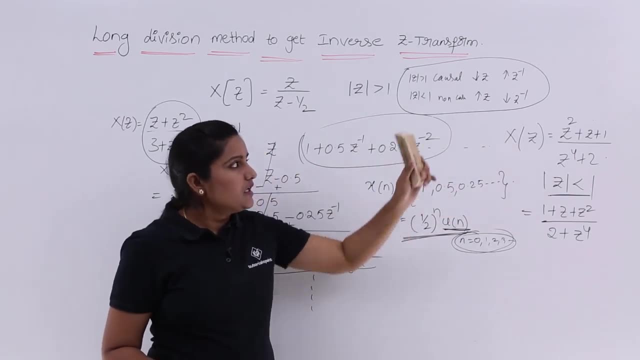 you need to consider descending powers of z, For example. system is non causal. how you can say system is non causal by this ROC. So if the system is non causal, then you can. you need to consider the ascending powers of z or descending powers of z, inverse that. 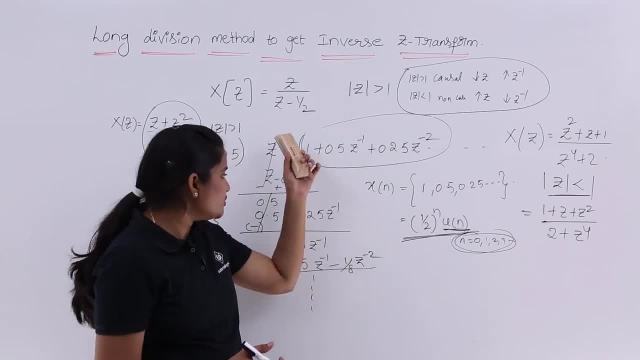 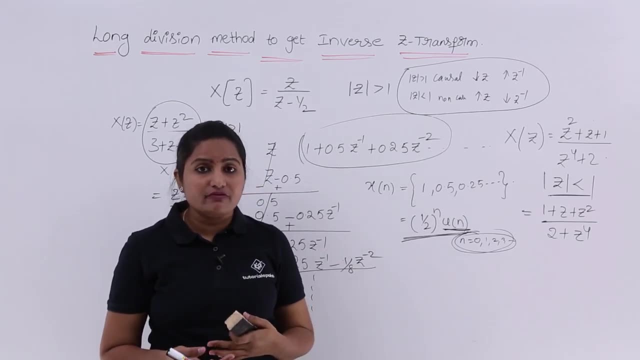 point is very important. after rewriting the equation, you need to perform like this. You are going to get the better result. In the next class we will discuss another method: partial fraction or a direct calculation method for inverse z transform.